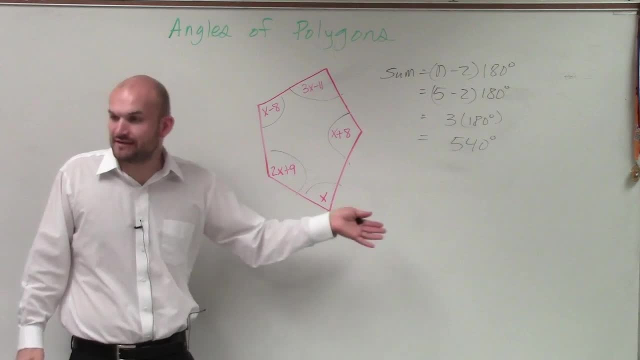 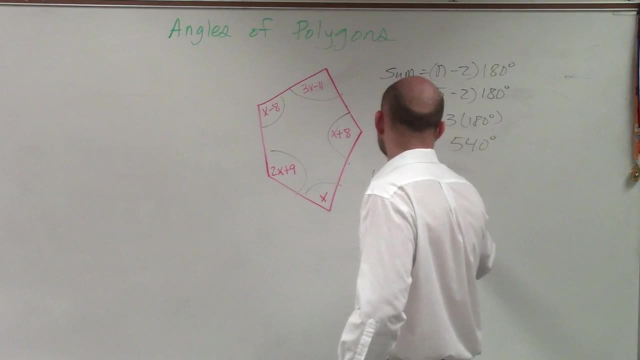 But you guys can see, these angles aren't just easy like numbers: 70 and 30 degrees, They're expressions. But that's OK. We can now just do x minus 8 plus 3x minus 11 plus x plus 8 plus 2x plus 9 plus x equals 540.. OK, Does everybody see what I did? 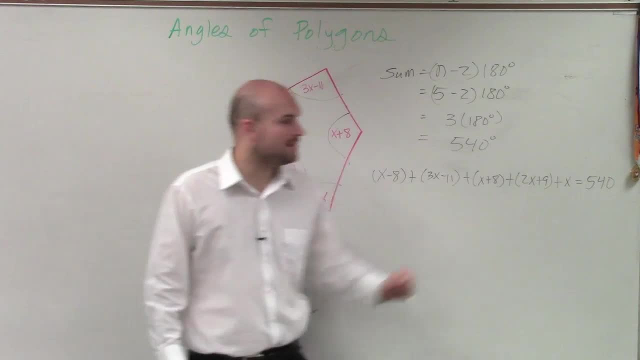 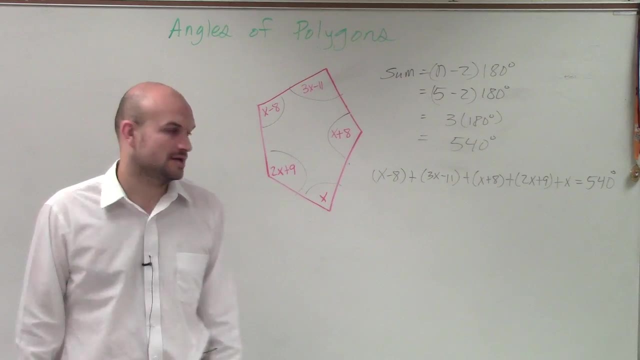 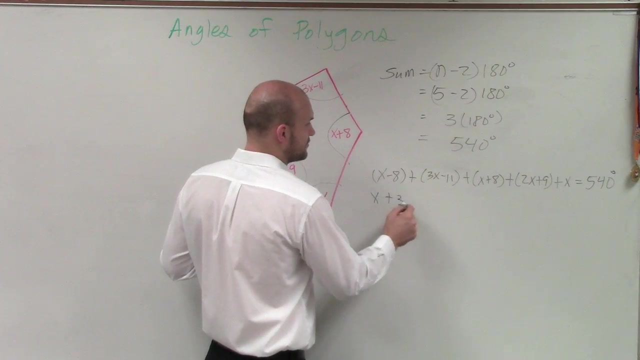 I took each one of these angles. I added them up to equal 540 degrees. Now I need to combine my like terms, So I'm going to rearrange this so I can add all the x's and then add all my numbers, So I can have x plus 3x plus x plus 2x plus x. 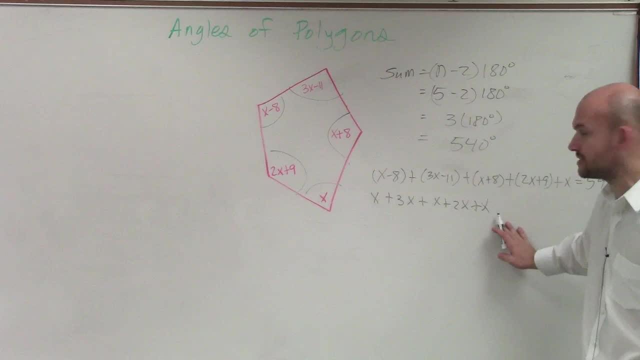 So all I did is now I rearranged the x's. You don't have to do this, but I'm just trying to help you guys out. And then I take all my numbers: Minus 8, minus 11, plus 8.. 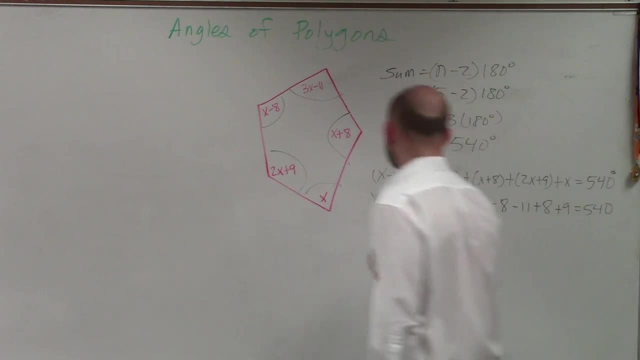 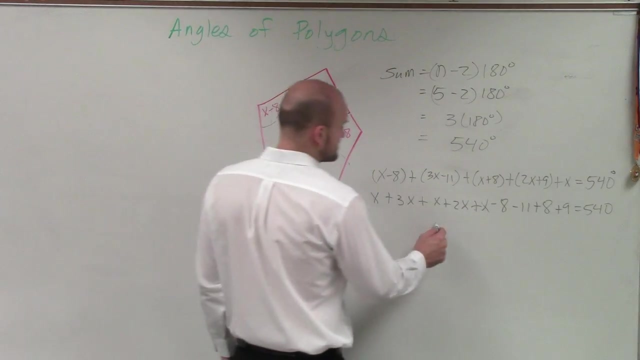 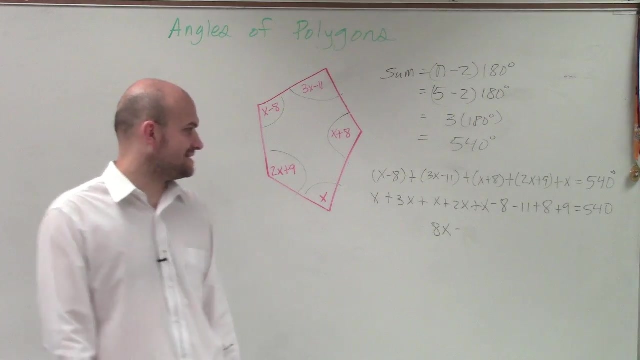 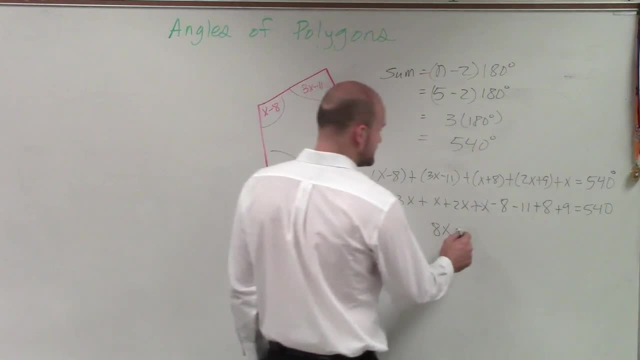 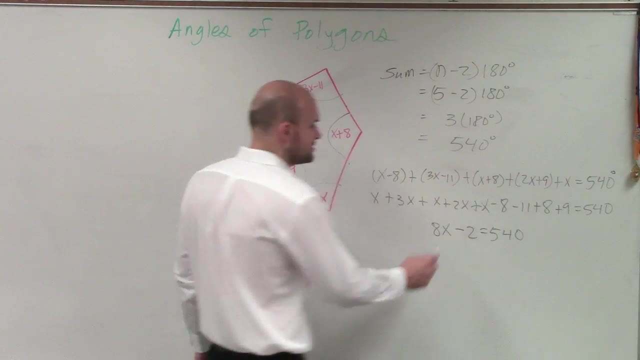 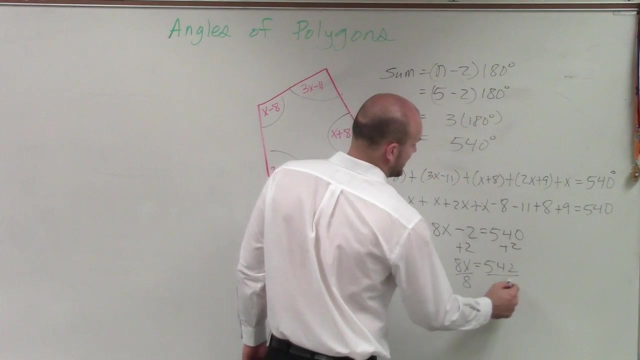 And then plus 9 is going to be a negative, And then plus 9 is going to be a negative. 2 equals 540.. Now to solve for x, I add 2.. So I have 8x equals 542.. Divide by 8.. 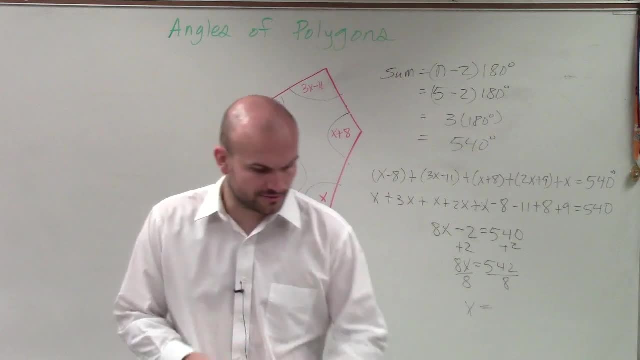 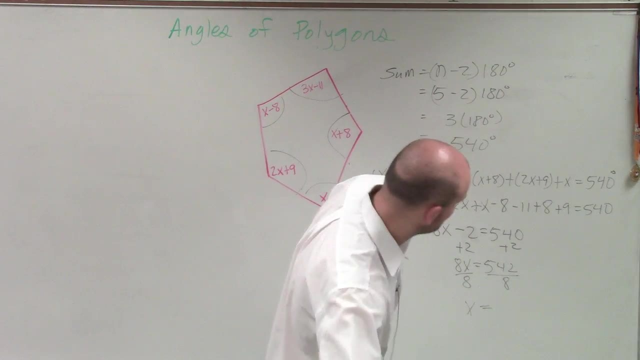 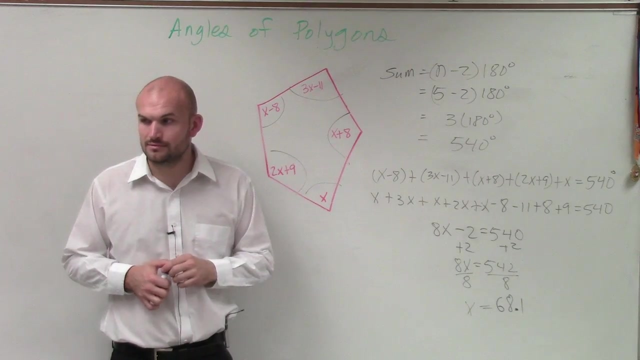 Divide by 8. x equals 542.. Huh, 68.1.. 68.1.. 68.1., 68.1.. So therefore, you guys can say: for all of these added in, your value of x has to be 68.1.. 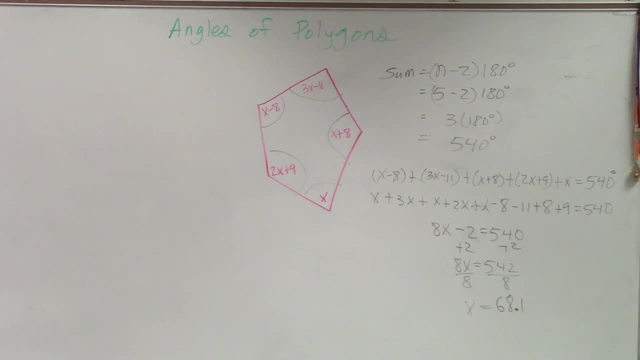 OK, And that's all you guys have to do Now, since I have.